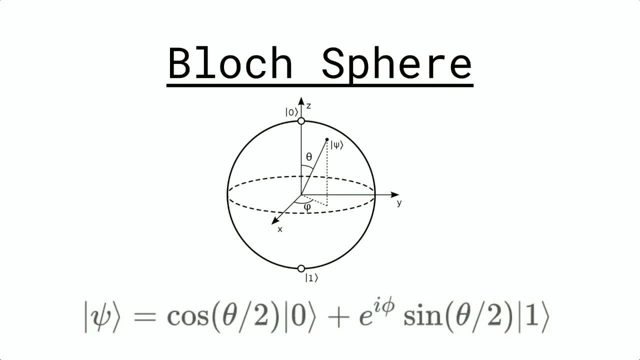 matrixes can get very big and difficult to work with. So what quantum computer scientists do is they like to represent qubits by this Bloch sphere, By representing a qubit by this equation. we get this nice understanding of a qubit by being able to. 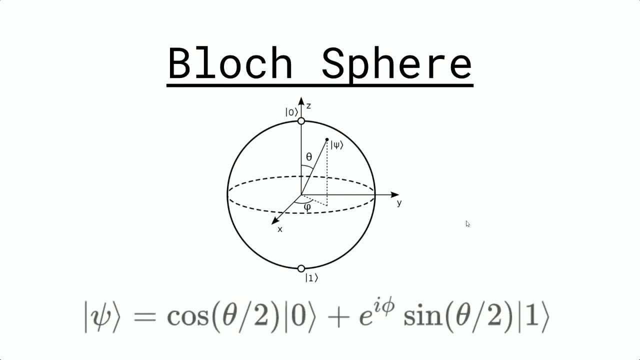 represent it by how it rotates within this sphere. So it has an x-axis, a y-axis and a z-axis, And the next quantum gates we're going to look at end up rotating the qubits around this axis. So these gates are what's called the Pauli gates. 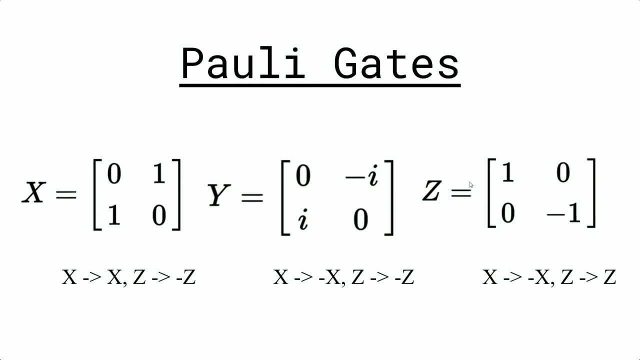 Now the Pauli gates. there's three of them. There's the, the x-Poli gate, the y-Poli gate and the z-Poli gate, And what these do is essentially end up rotating the qubit around either the x-axis, 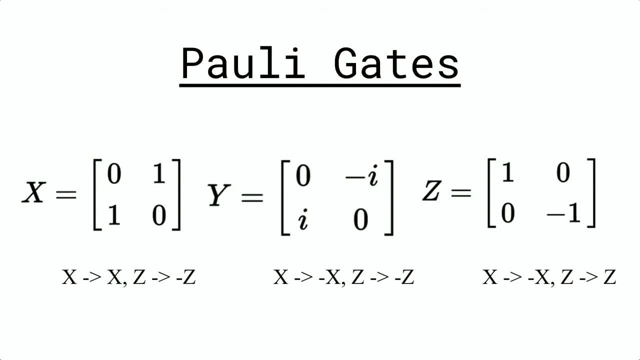 the y-axis or the z-axis And we can see the actual rotations that they make right here. So flipping a qubit around the x-axis keeps the x-axis the same but makes the z-axis the inverse of itself. So let's look at that. on the, the quantum systems, 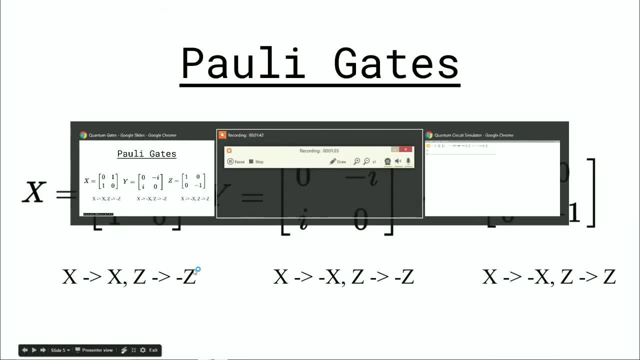 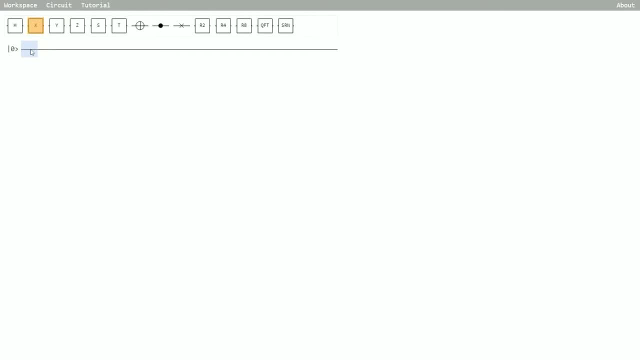 So let's look at that on the quantum systems. So let's look at that on the quantum systems, quantum simulator. So if we apply a x-gate right here, this is what's called the not-gate, the poly-not-gate. So when we run it, we see that it inverses the state of 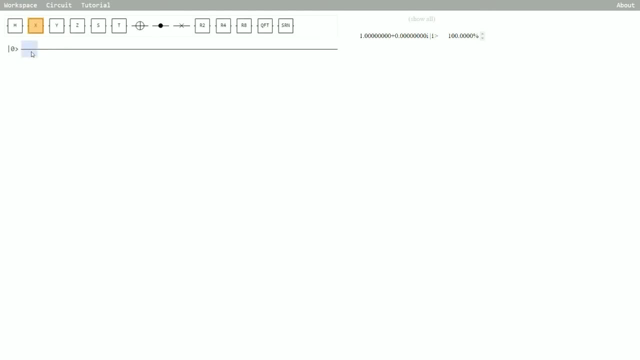 the qubit to be 1.. Now, when we do this with the y-gate, we see that the same thing occurs. The state is still that you're measuring it, it's still going to be in a 1, especially because we haven't put it into superposition yet. We can see that the 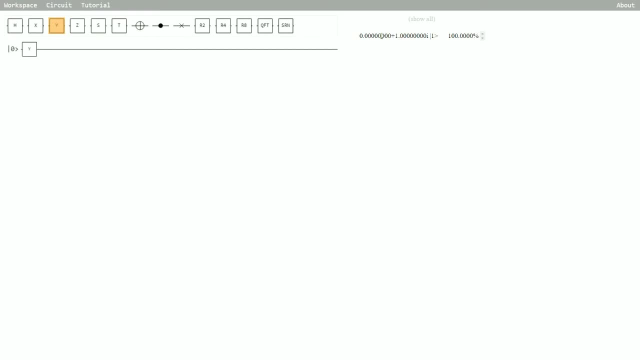 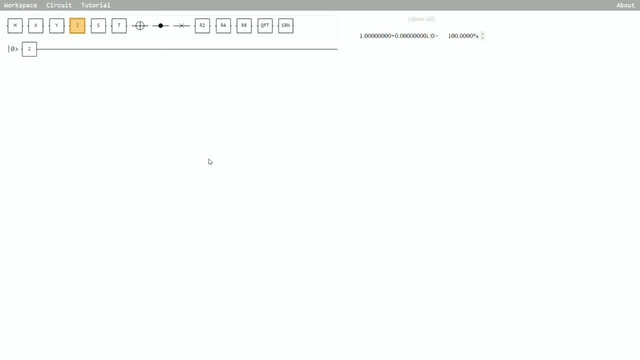 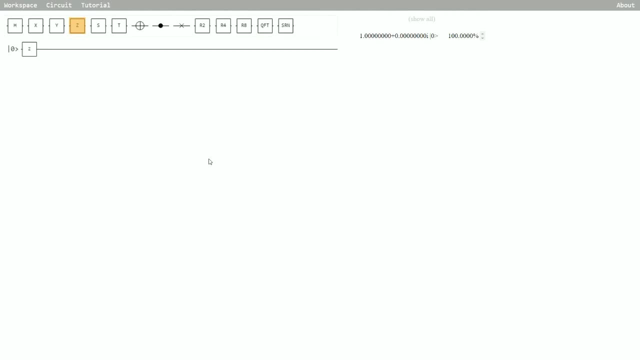 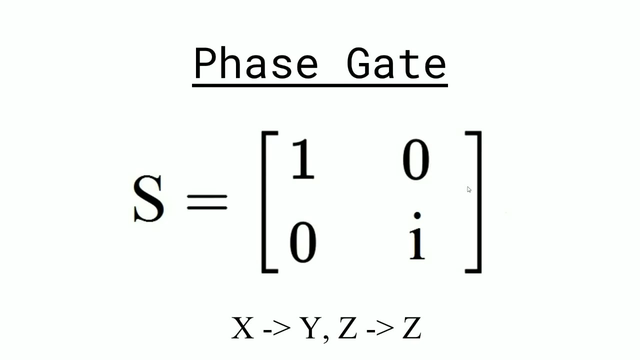 we will be able to make calculations as a result of that. so the next gates we're going to look at are called the phase gate and the phase rotation gates, and what these do is they leave the basis state of a qubit unchanged, which is zero, but they map. 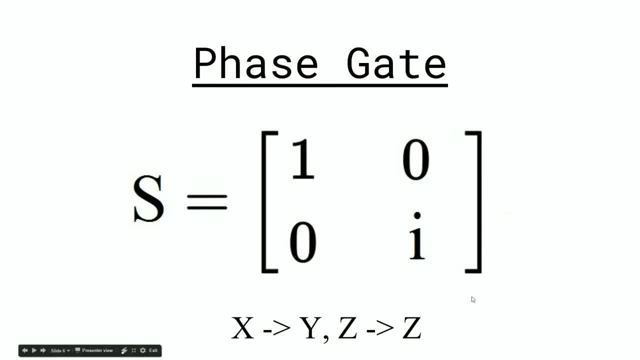 a, a complex number to the one value, which has the effect of leaving the expectation value of a qubit unchanged, but allows us to to rotate a qubit in the block sphere or change the phase of it, and this allows us to create complex superpositions after we put qubits through. 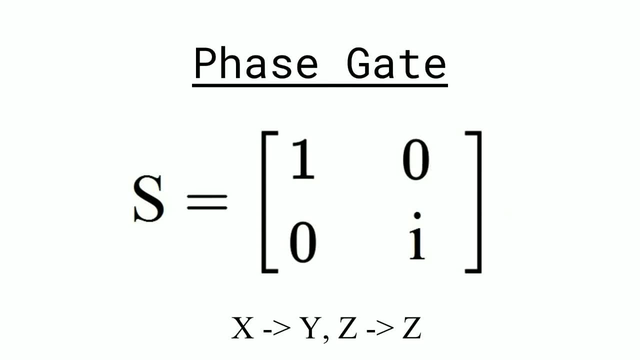 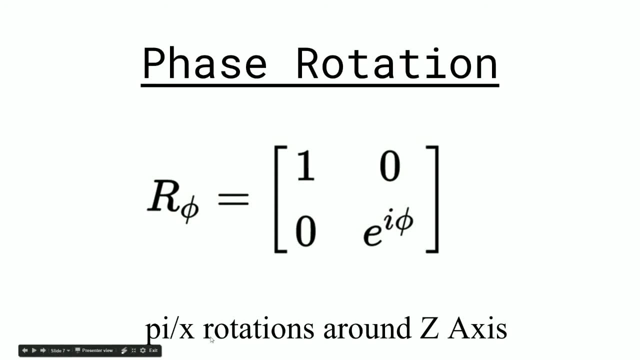 through the hadamard gate. so here's the matrix for a phase gate and here's the matrix for a phase rotation gate, where we're able to to rotate a qubit in any ratio we want, so we could rotate it half a rotation or a quarter. 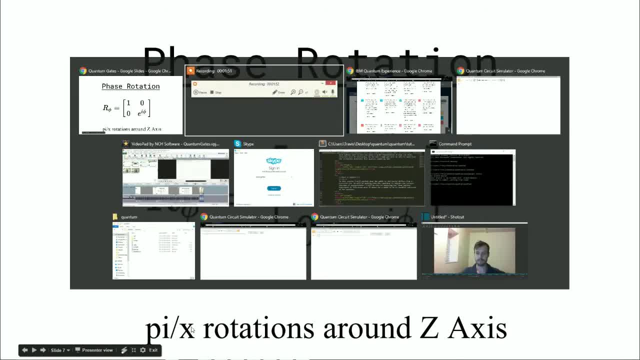 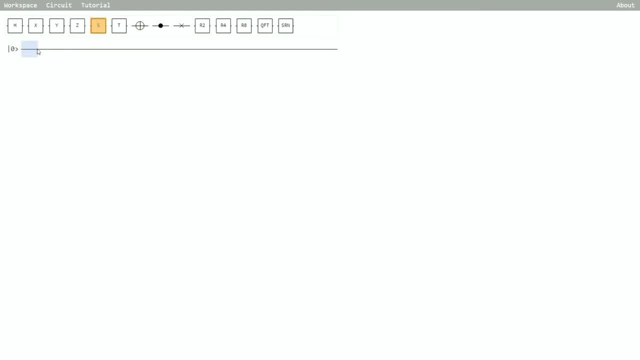 rotation or an eighth rotation. so let's see an example of that on the simulator. so if we apply a a phase gate to to this qubit, we see that its expectation value is 100. this, this phase gate, doesn't change that at all. but if we are now to apply a hadamard gate, 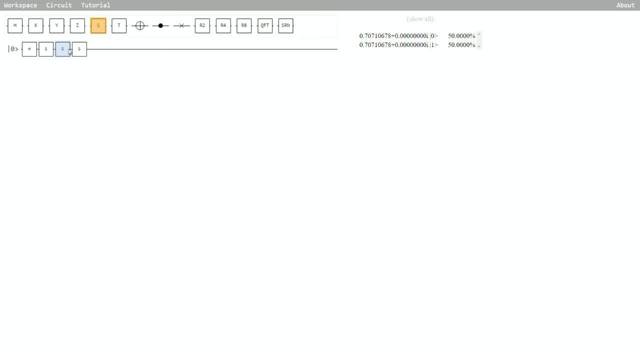 and then apply the phase gate, we still see that the, the expectation value, doesn't change. but as we apply these phase gates, we see that this complex number is changing and and this represents the position of the qubit within the block sphere. so if we, if we apply these, 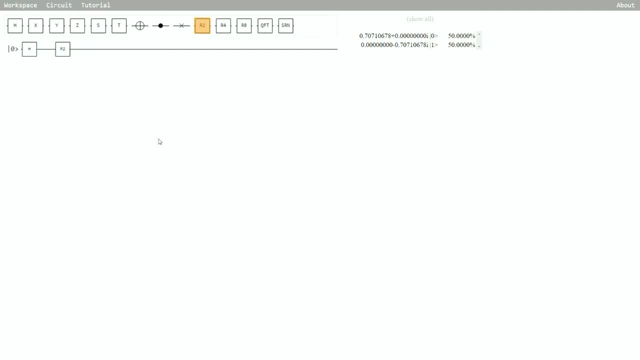 phase rotation gates, which are the, the ratio gate which I was talking about earlier. here's the, the half rotation. we see that, once again, the complex numbers are changing, but the expectation value isn't, and we can do the same for the quarter rotation and the eighth rotation as well, and you can see how. 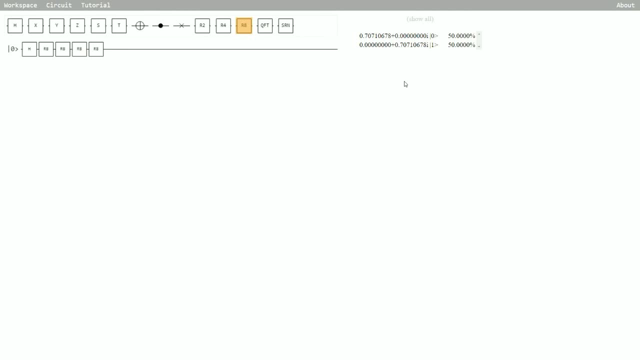 this is changing the complex number of the qubit, which is representing how it's rotating in the block sphere, and by changing its phase for more complex algorithms, we're able to solve different equations, as as we'll see in upcoming videos, the control- not gate- is a bit different from the other quantum gates we've been 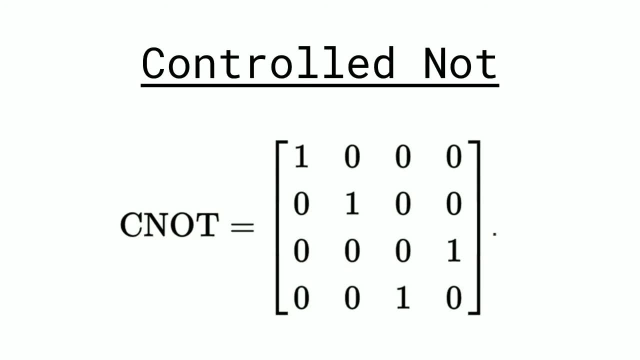 looking at, since it requires as input two qubits and it outputs two qubits as well, since all quantum gates have to be reversible- and how it works is it flips the bit of a second qubit, so it knots it, depending on the value of the first. 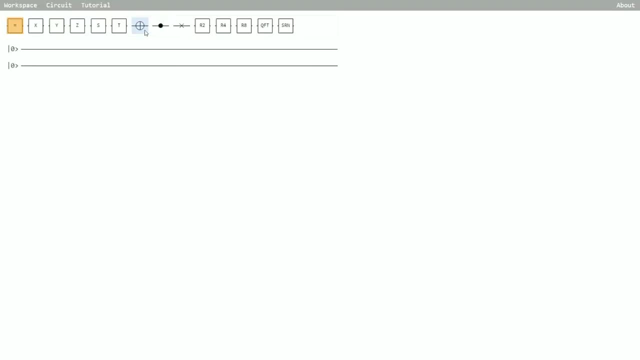 qubit. so if we run this on the, the quantum simulator, we put a control, not gate, in like so, and we we run this, we see that the output is 0: 0 because the indicator value for this qubit isn't on and it isn't telling the second qubit to to. 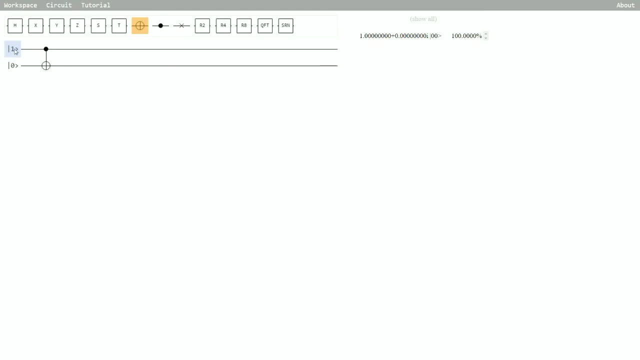 flip. but if we now turn the indicator cubit to one and run it again, we see that indeed, this bit has now been flipped from 0 to 1, and if we turn this qubit to 0 and run it again, we see once again it. 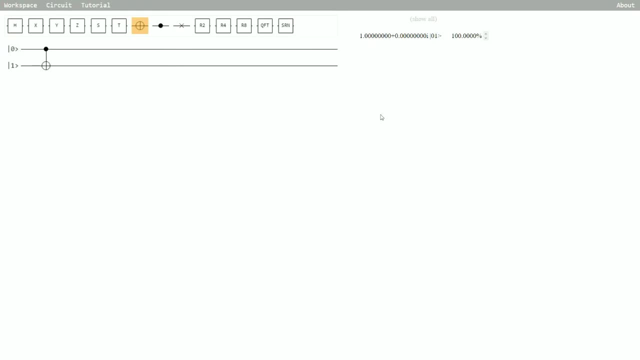 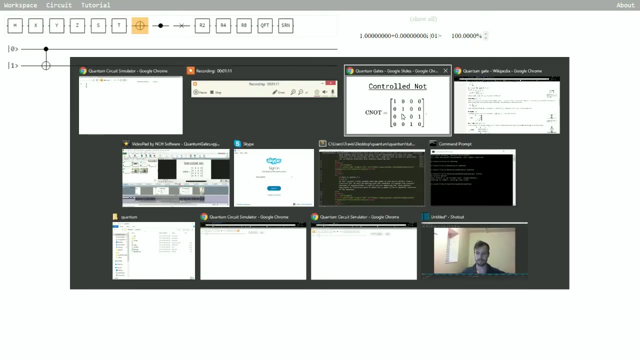 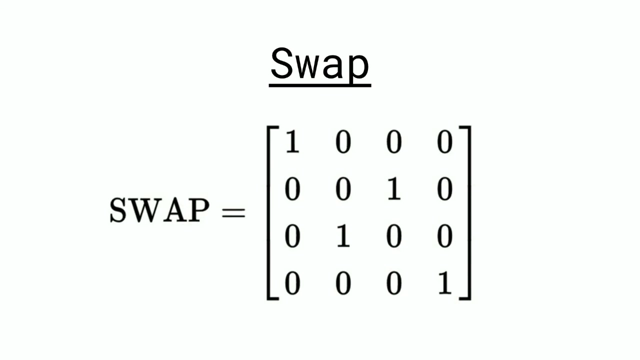 flipped And if we turn the indicator value on we see that now the bit no longer flips. So that's how a controlled NOT gate works. And the next gate, a swap gate, just like the controlled NOT gate, also takes as input two qubits and outputs two qubits. And how it works.